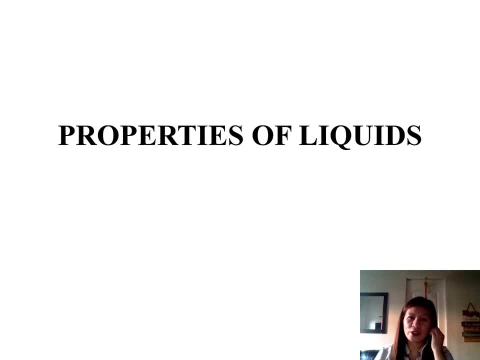 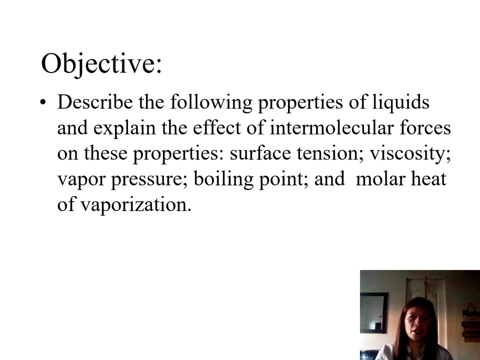 Good day class. welcome again to our general chemistry 2 class. So for this video we're going to discuss about properties of liquids. For the objective: describe the following properties of liquids and explain the effect of intermolecular forces on these properties: Surface tension. 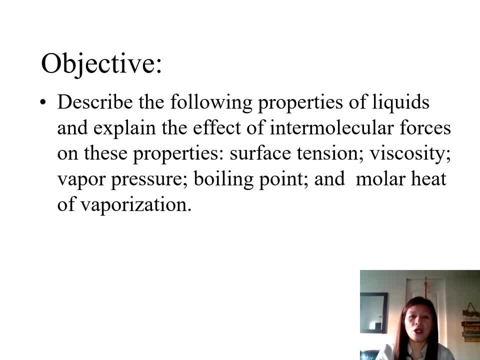 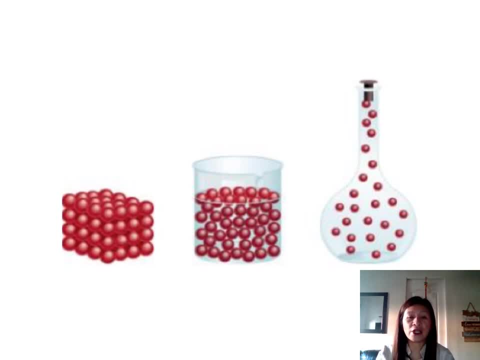 viscosity, vapor pressure, boiling point and molar heat of vaporization. In the last video we distinguished among the three states of matter in the light of the kinetic molecular theory, So we distinguished them in terms of properties such as volume, density, spaces between particles. 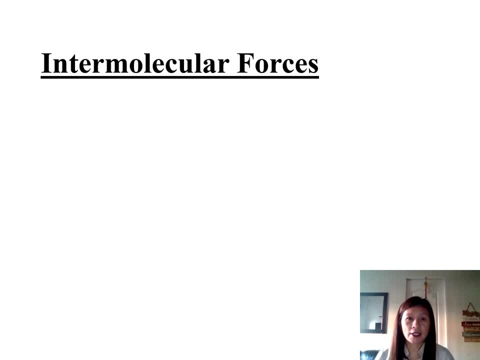 and forces. We also discussed the different intermolecular forces, the forces that are responsible for the formation of the different states of matter. So we have the distribution or London forces, the weakest of all intermolecular forces, which exists in non-polar molecules. 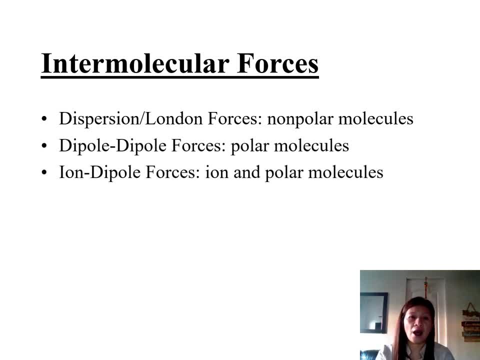 the dipole-dipole forces in polar molecules, ion-dipole forces between ion and polar molecules and hydrogen bond, the special dipole-dipole forces that exists between hydrogen of one molecule and an electronegative fluorine, nitrogen or oxygen of another molecule, And in this particular 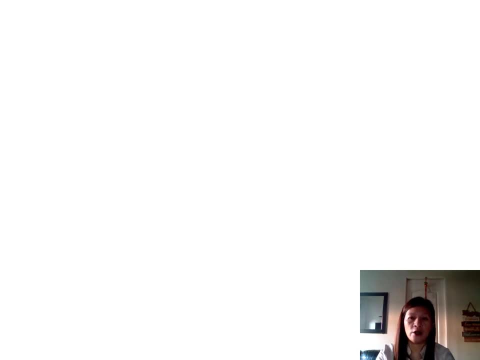 and which is also strongest among the four intermolecular forces. So as a review, let's determine the type of intermolecular forces between the molecules of the following substances. Number one: benzene. Benzene is a nonpolar substance or molecule. So for nonpolar molecules it's exclusively dispersion. Dispersion is a result of polarizability of molecules. Polarizability is the ease to distort a molecule, So nonpolar molecules are highly polarizable. That's why dispersion, which is also the weakest of all the intermolecular forces, exists between the molecules. 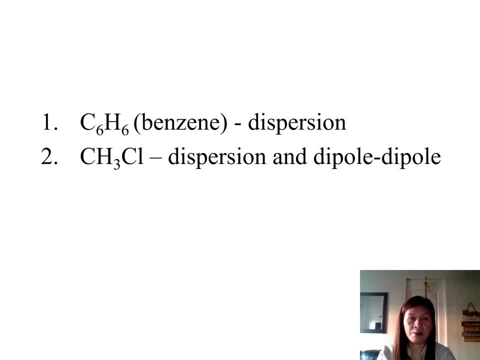 Chloromethane or methyl chloride is a Nonpolar molecule, So definitely it's a dipole-dipole, because for polar molecules the type of intermolecular force is dipole-dipole. But since dispersion is a result of polarizability of molecules, dispersion also exists in all molecules, between all molecules. 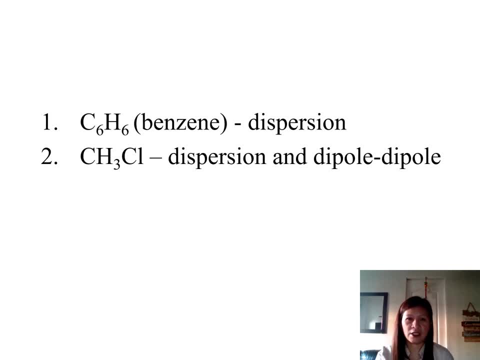 So dispersion is another type of intermolecular forces that exists between chloromethane. Another is phosphorus trifluoride. Phosphorus trifluoride, like number two, is also a polar molecule and therefore another dipole-dipole. 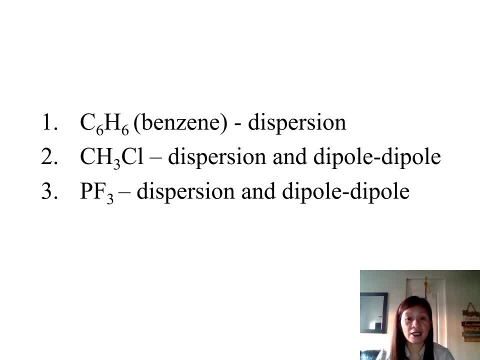 But again, dispersion exists in all types of particles and therefore dispersion is another IMF between the particles of the substance. Sodium chloride, it's dispersion, Again dispersion- and ionic And carbon disulfide Sodium chloride is a nonpolar and therefore dispersion. 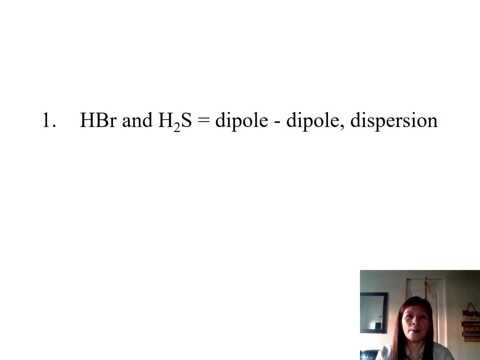 What about between the following substances: Hydrogen bromide and hydrogen sulfide are both polar, So therefore between them it's dipole-dipole. But again, dispersion exists in all types of molecules or particles and therefore dispersion is also existing between the particles. 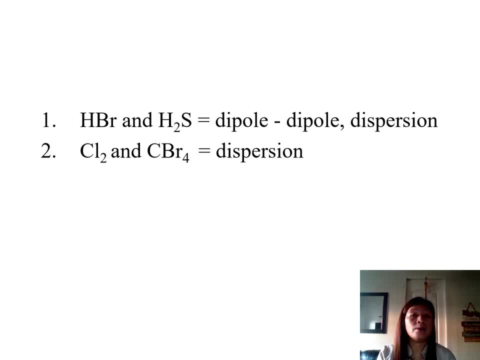 So dispersion exists in all types of substances. Number two is diatomic molecule chlorine and carbon tetrabromide. Both are highly polarizable, Both are nonpolar and therefore exclusively dispersion. Another diatomic molecule, iodine and an ion nitrate. 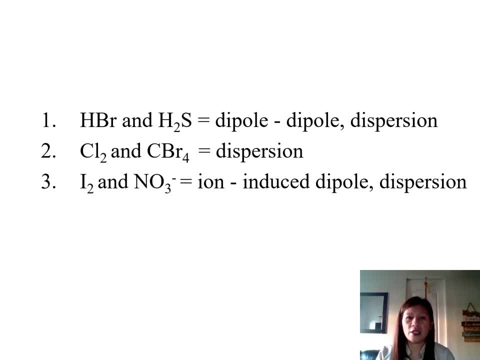 So this is ion-induced dipole dispersion Induced dipole because the neighboring ion is ion-induced. So this is ion-induced dipole dispersion Induced dipole because the neighboring ion is ion-induced And this ion will cause the nonpolar iodine molecule to be induced. 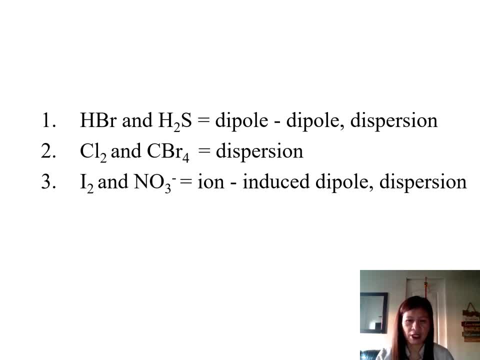 To become an induced dipole And therefore the type of force is ion-induced dipole and also dispersion. Another is ammonia and benzene. Ammonia is polar, Benzene is nonpolar And therefore dipole. Dipole because 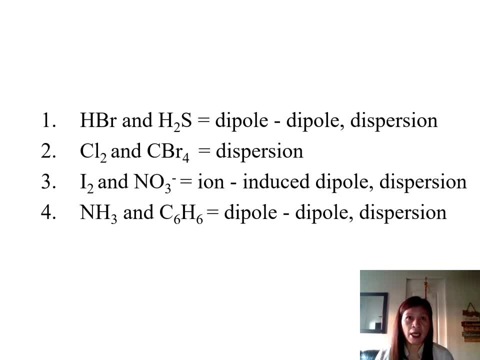 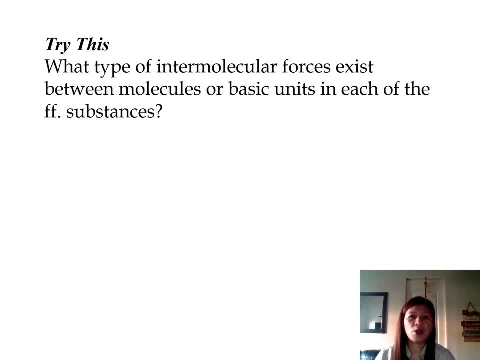 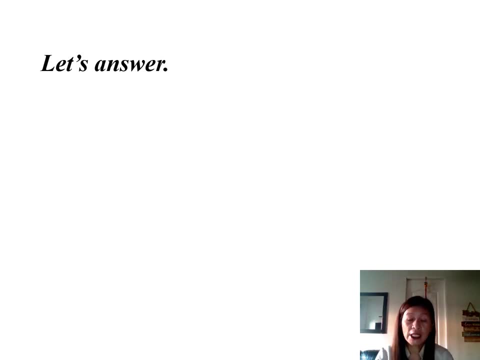 Because, Because, Because, Because, Because, Because, than dipole-dipole. If it has hydrogen and nitrogen, fluorine and oxygen attraction or bonding, then a special dipole-dipole, which is hydrogen bonding, And if there is presence of 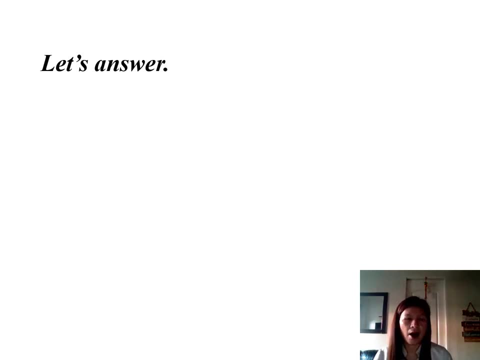 ion and another dipole, or highly polarizable, nonpolar, then it will be ion-induced dipole or simply ion-dipole forces. So it depends on the polarity of the molecule. You can determine the type of intermolecular force between the particles. Number one: water. Water has hydrogen. 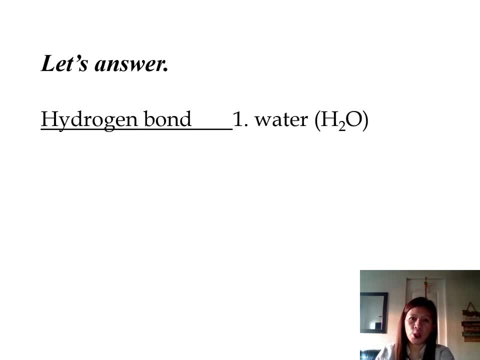 oxygen atoms in each molecule. So since there is hydrogen and oxygen, a hydrogen bond is exclusive with oxygen, nitrogen and fluorine. So hydrogen bond is a result of the attraction between hydrogen of one molecule of water with oxygen of another molecule of water, So that 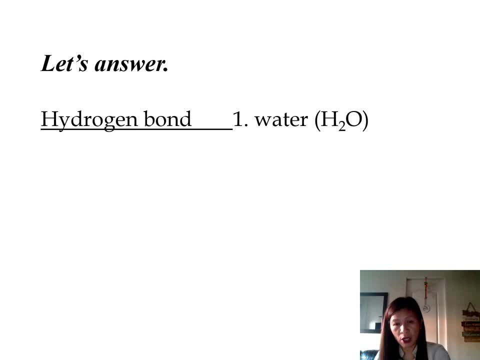 bonding between hydrogen and oxygen of another molecule is called the hydrogen bond, a stronger dipole-dipole force. Ethanol also has oxygen in the molecule. So if there is oxygen in the molecule it also is possible to form a hydrogen bond between oxygen of one molecule of ethanol and. 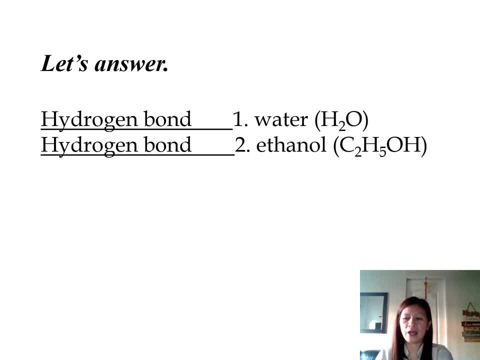 hydrogen of another molecule of ethanol. So this is another hydrogen bonding or hydrogen bond, And another oil With the general equation C, sub n, H, sub n, O, sub n. This is a nonpolar molecule and therefore dispersion. So again, it depends on the type of molecule whether 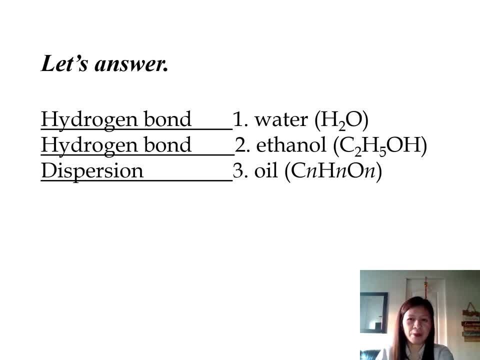 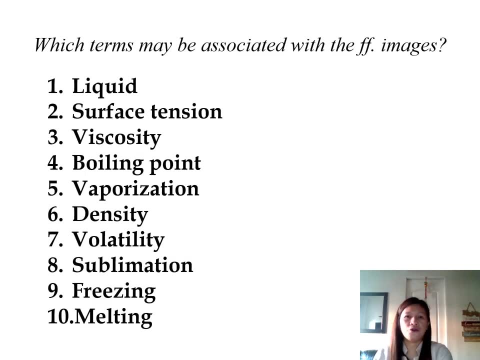 polar or non-polar, you can tell or determine, identify the type of intermolecular. for another exercise, let's have the following terms. these terms are either the properties or associated with the properties of liquid. so again, our topic in this video is properties of liquid. so i'm going to show you some images you associate the following terms with: 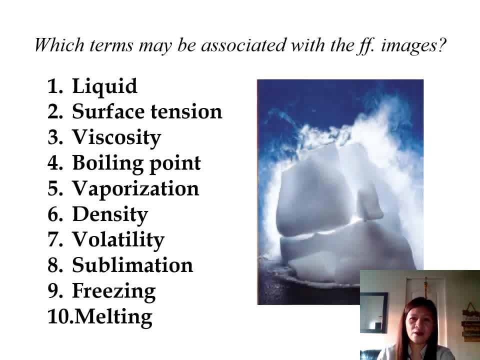 each of the images, number one: we have this picture, so what? which terms can be associated with the picture? so it can be liquid, yes, we can also associate vaporization, because you see formation of gas. we can also associate density, because you have fluid and solid. we can also associate volatility, for as 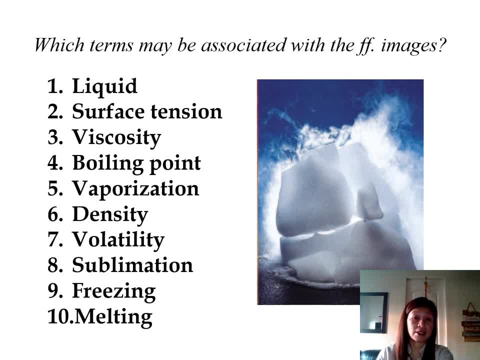 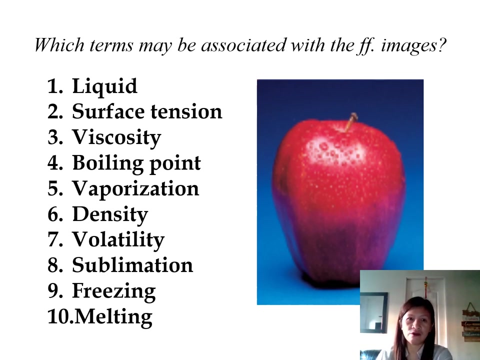 long as you have liquid, what else? sublimation, because solid seems to turn to gas. freezing, because this seems to be a frozen liquid, and melting, because this is a frozen liquid, it may be assumed to be melting. another is this apple. we can associate liquid because you see beads of liquid on the surface of the apple. 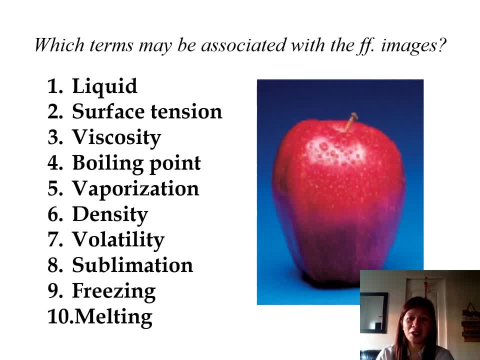 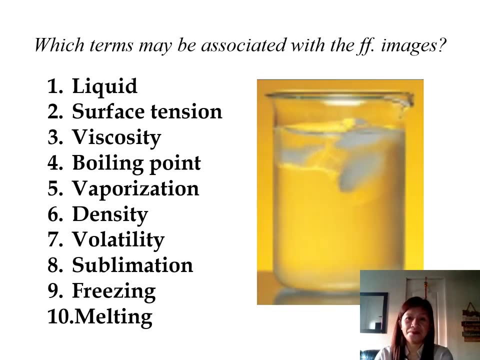 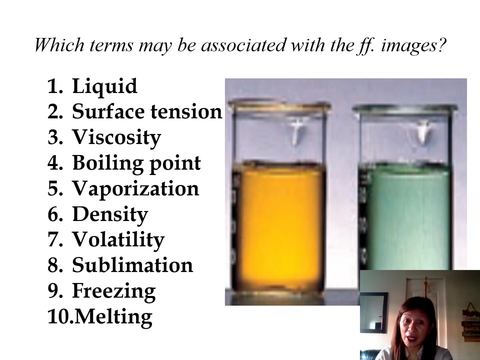 we can also associate surface tension, if you know the what, what explains the formation of beads on the surface. we can also associate um density- yeah and okay, we have liquid here, we have um melting, freezing density. of course, volatility as well. we can also associate vaporization. we can associate here liquid viscosity, boiling point, density, volatility also. 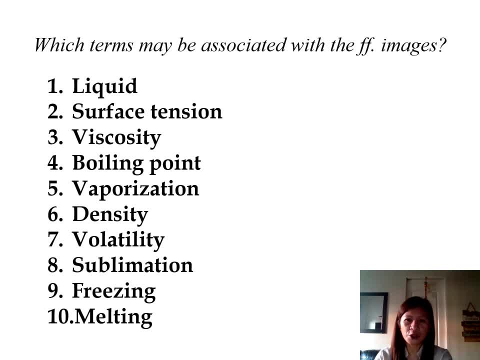 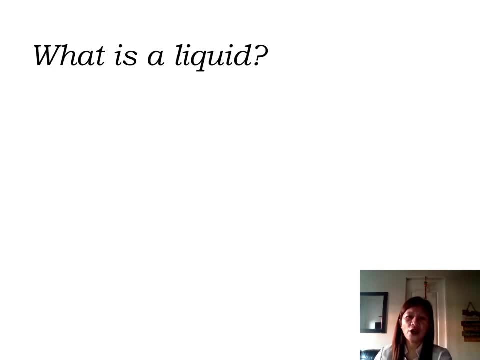 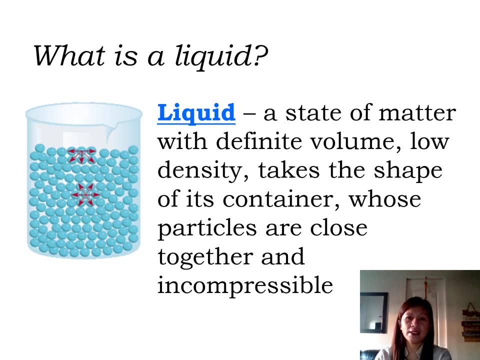 melting, freezing also, so almost all the terms can be associated with each of the images that the. Let's now define a liquid. What is a liquid? A liquid may be defined as a state of matter with definite volume, low density. takes the shape of its container, whose particles are close together and are incompressible. 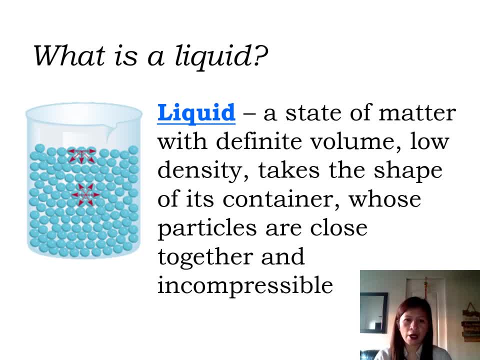 Because of the limited spaces between particles, they are incompressible. Particles are also in random. They are not closely packed. The container also contains the molecules. Because of the loose attraction, particles may have the ability to flow and break away from the attraction. 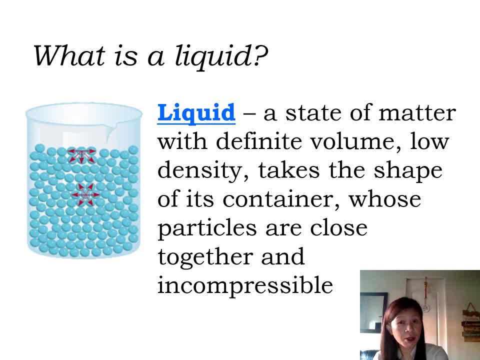 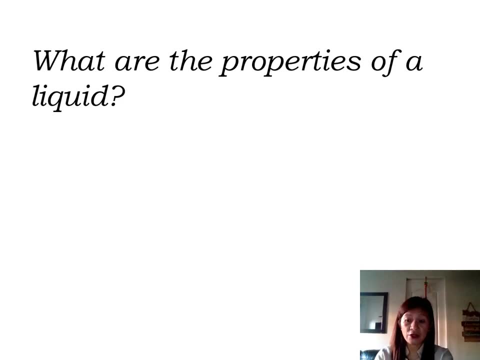 What else? Whatever the volume of the container, the shape of the container, they will be taken by the liquid. So those are some of the characteristics of the liquid As shown in this illustration. Now, what are the properties of a liquid? Number one is surface tension. What is surface tension? 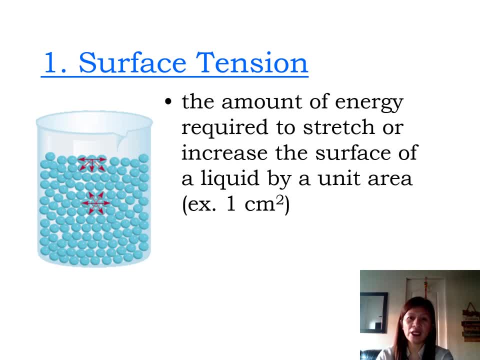 It is the measure of the amount of energy required to stretch or increase the surface of a liquid by a unit area, For example by one square centimeter. It can also be defined as the resistance of a liquid to increase. So the more resistant a liquid is to stretch its surface area, the higher its surface tension. 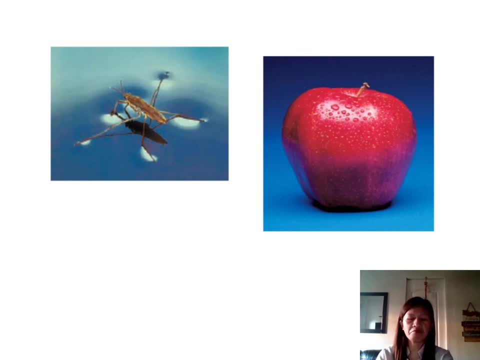 So we have here the following images. So number one: you see a water strider being able to walk on water. Water has oxygen and hydrogen. Water has oxygen and hydrogen. So the type of intermolecular forces is a strong IMF, which is hydrogen bond. 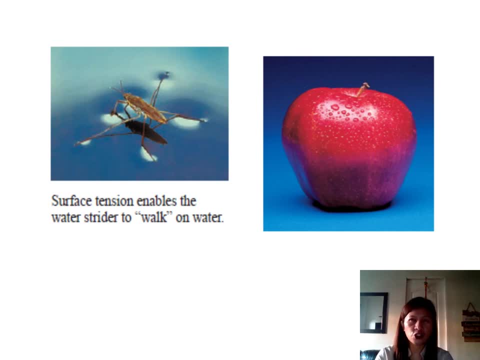 Since there is a strong attraction, intermolecular attraction, between water molecules, it is not easy to increase the surface, So it requires higher energy to increase the surface area. And because the insects are not heavy, or, for example, in this example, in this image, the water strider. 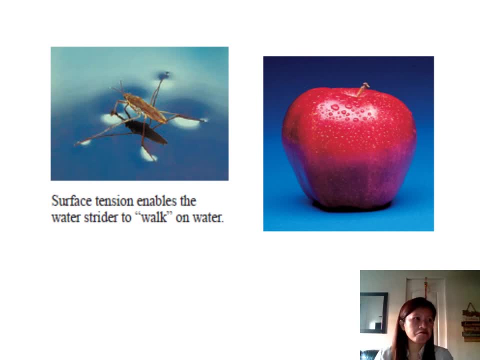 the weight of the insect or this animal is not sufficient enough to break the chemical bond that exists between the water molecules. So the water is resistant to increase in its surface area. So that's the reason why insects are able to walk over. So that's the reason why insects are able to break the chemical bond that exists between the water molecules and the water particles. 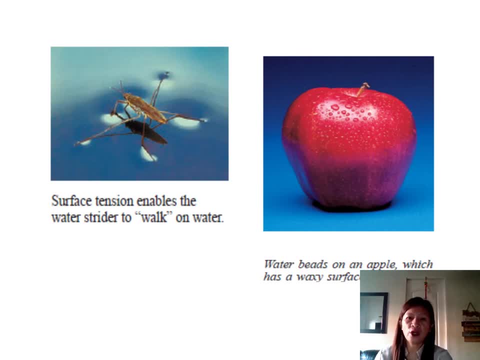 So the water can do that. they are able to do that. Another reason is the formation of water beads on an apple which has a waxy surface. So again, water umm, ummm. apple has a waxy surface. 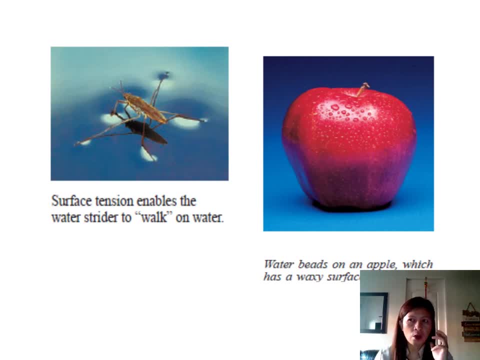 Since ummm, ummm wax as- or-or-or-or-or-or, or-or-or-or-or-or-or-or-or maybe assumed as oil is insoluble in water, They- they do not reach the surface- have different polarity. okay, water is polar, oil is nonpolar, so they will not. 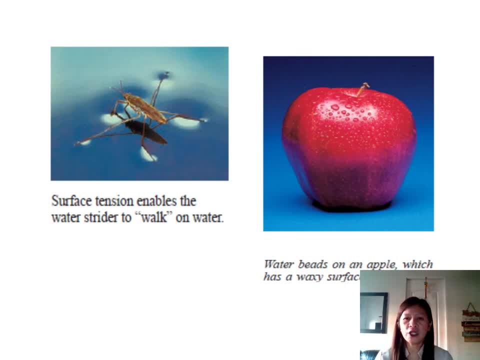 mix together. so that's the reason why water-heel foams beads: because water molecules at the surface of a liquid are being pulled towards inward. rather, water molecules are being pulled inward by molecules below the surface, below the surface molecules. that's why water molecules tend to form beads on the 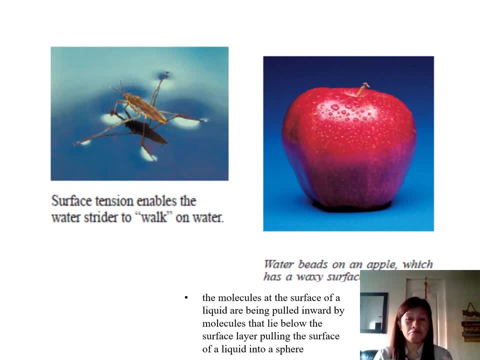 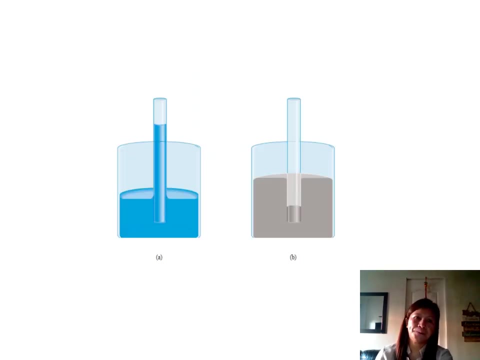 surface of a waxy apple. okay, so that's what makes the water molecules form beads on the surface of the uh apple. okay, we have here, uh, two liquids. letter a is water and b is liquid mercury. so, as you can see, by capillary action there's rising of the liquid in the narrow tube. but what is the difference? 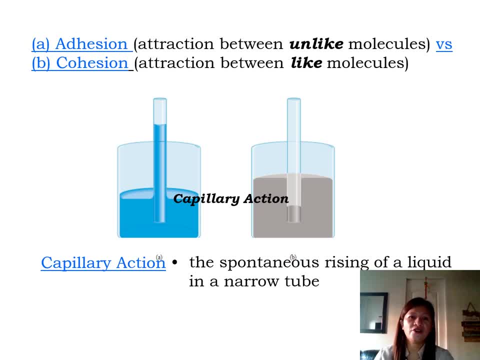 between the two. let's take note of the two forces. in the following we have adhesion and cohesion. adhesive forces are the attractions between unlike molecules, cohesion between like molecules. so where is cohesion and where is addition here? cohesion is the force between water molecules. also, creation is the force between particles of liquid mercury, so between 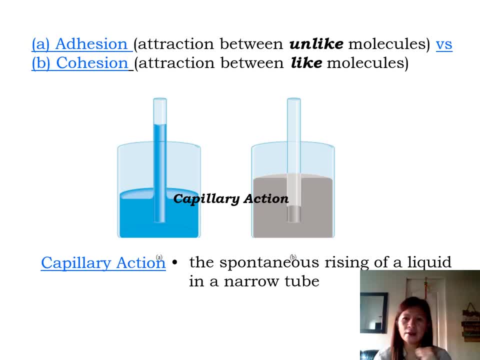 the like molecules of water and liquid mercury. its cohesive force, adhesion, is between the water and the glass, it's between the mercury and the glass. so that's adhesion, unlike attraction between, unlike molecules. notice the meniscus. meniscus can be concave, like a. 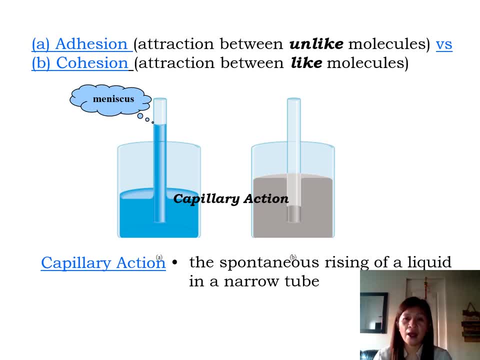 like what forms here in water? or convex as what forms here, with mercury back, if fucker. or on concave meniscus and concave convex meniscus. this happens con con cave meniscus, as in water happens when the adhesive force is greater or stronger than the cohesive. 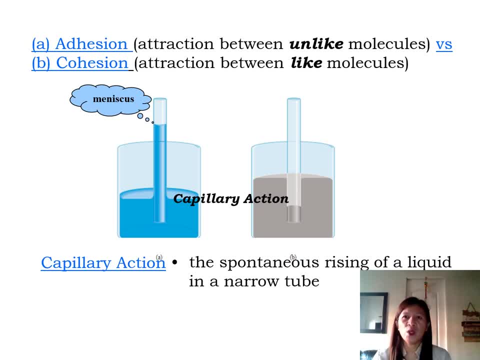 water. On the other hand, between the molecules of, or between the particles of mercury, mas strong yung cohesive pores, yung attraction between the mercury particles kesa dun sa attraction between the glass and the mercury particles. So that's the reason why the meniscus forms convex. Mas mababa rin yung pagakyat ng liquid, kasi nga mas attracted yung mercury particles dun sa other mercury particles, kesa dun sa glass. 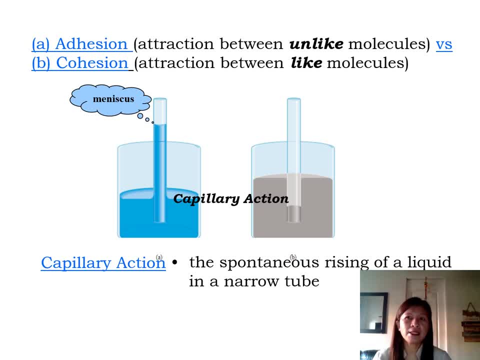 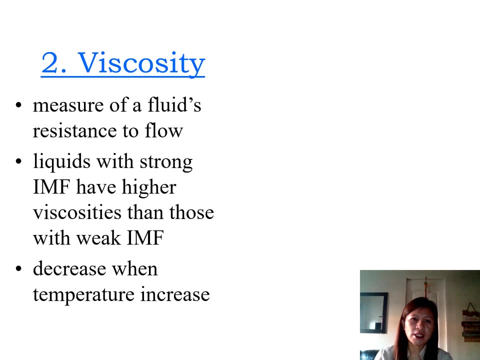 Unlike dun sa water, mas malakas yung attraction ng water dun sa glass kesa, dun sa glass Kesa sa attraction ng mga water molecules with one another. Another property of liquid is viscosity. Viscosity is the measure of a liquid's resistance to flow. 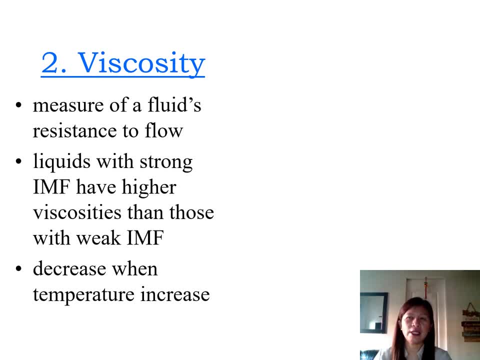 So the more resistant to flow, the higher the viscosity. So it's like the behavior of water, the ability of water to flow and the ability of oil, for example, to flow. When compared, alam naman natin na mas mabilis mag-flow ang water kesa sa oil, Mas resistant ang oil. 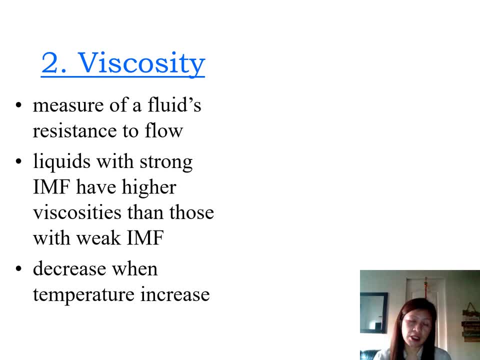 Therefore, the more resistant, the higher the viscosity. So we can say, we can conclude that oil is more viscous than water. Liquids with strong IMF have higher viscosities than those with weak IMF, Mas malakas yung attraction between the mercury particles and the mercury particles. 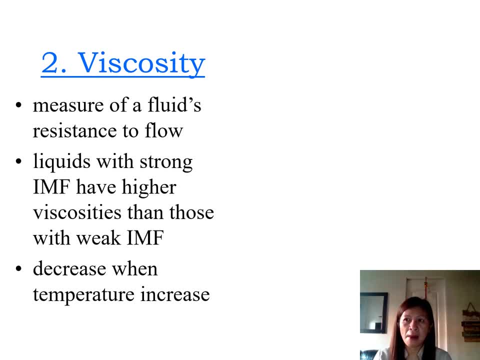 Attraction between particles mas held strongly sila by themselves, So mas resistant sila to break away from the attraction and flow. Hindi katulad nung weak yung attraction, mas madaling mag-break away from the bond and mag-flow freely. 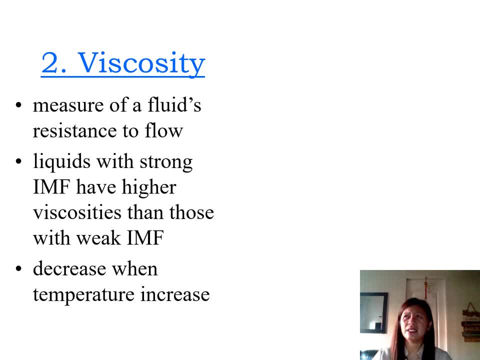 Also, viscosity decreases when temperature increases. It's like magma. Kung ma-imagine natin yung magma pagkalabas sa crater, mainit mas mabilis yung flow Once na nag-cool siya, habang lumalamig siya, mas bumabagal siya. 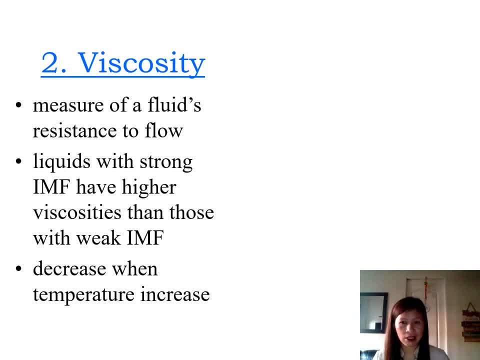 So increase in temperature decreases viscosity, Decrease in temperature. mas mababa yung temperature Mas malamig, mas mahina, Mas mabagal, din mag-flow, Mas highly viscous. So that's how we refer to viscosity. 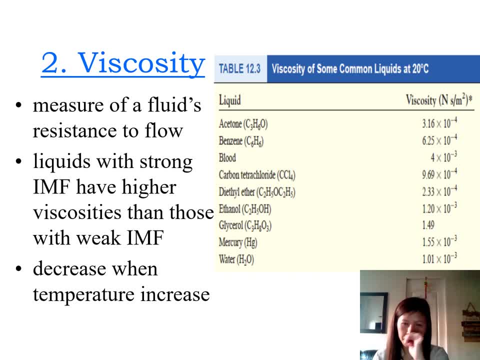 Let's compare the viscosity of some fluids. here We have acetone and let's have blood. Blood has viscosity of 4 times 10, raised to negative 3. When compared to acetone, If we are going to make use of some typical liquids- salimbawa, ang, water and alcohol, 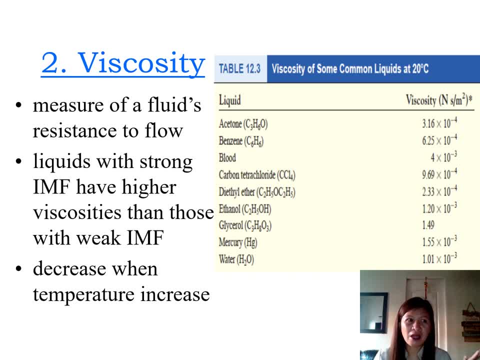 alam natin na madaling mag-evaporate ang alcohol. Of course we have established that oil is more viscous than water by observation: Mas mabilis mag-flow ang water, So less viscous siya kesa sa oil. 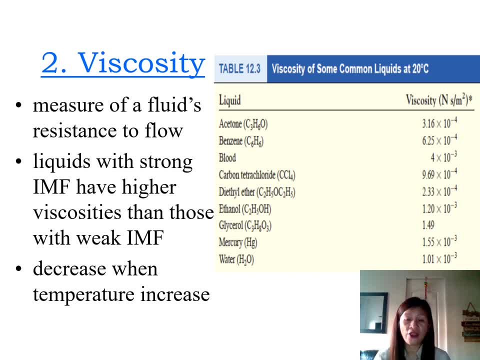 Oil is more resistant, Mas mabagal mag-flow And therefore higher viscosity. When comparing, for example, acetone and water, same thing, Or alcohol and water, Hindi natin iniiwan, basta ang alcohol or ang acetone ng open sa air. 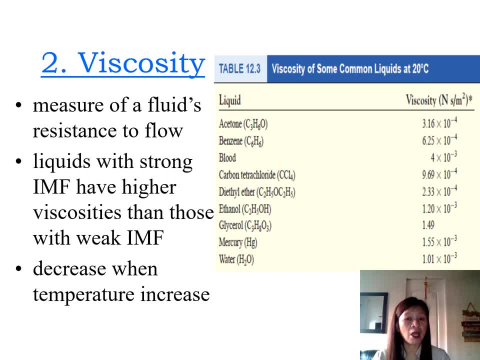 Kasi alam natin na after some time mauubos siya, Kasi mas mabilis mag-evaporate, Kasi mas mahina yung attraction between parts, Mas mabilis mag-break away from the chemical bond. 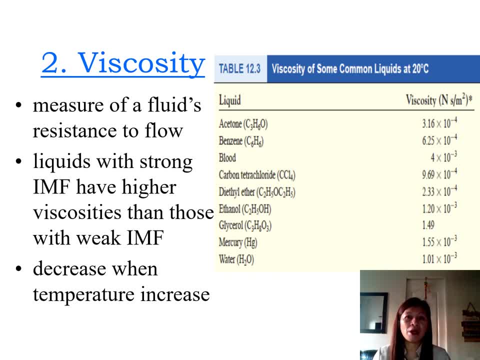 And therefore mas mabilis siyang mag-flow or mag-break away. So the strength of intermolecular force has something to do with, or viscosity also has something to do with, the strength of iron. The stronger the IMF, the intermolecular forces, the more difficult to break away from the chemical bond. the more viscous is the liquid. 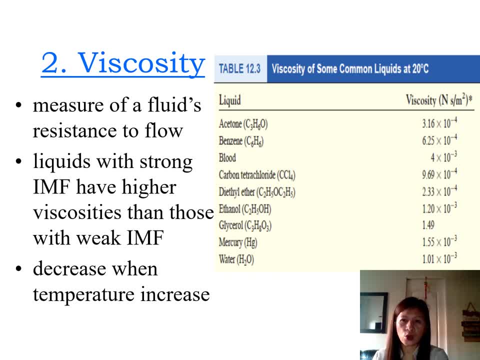 So compare this. When comparing blood and acetone, we have blood 4 times 10 raised to negative 3.. This is much greater than that of acetone, which is 3.16 times 10 raised to negative 4.. The difference in the exponent negative 4 is smaller than negative 3 of blood. 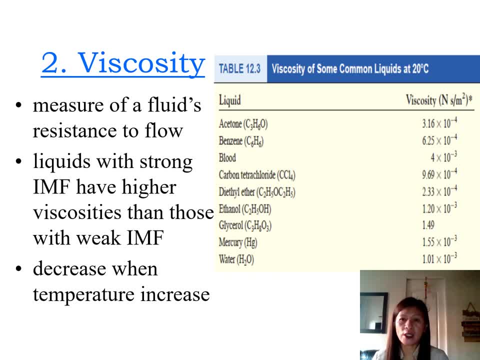 Therefore blood has higher viscosity than acetone. We also observed na mas malapot talaga ang blood, Kasi sa acetone Di ba meron nga tayong saying na blood is thicker than water And on that note mas malapot in layman's term, mas malapot, mas viscous. 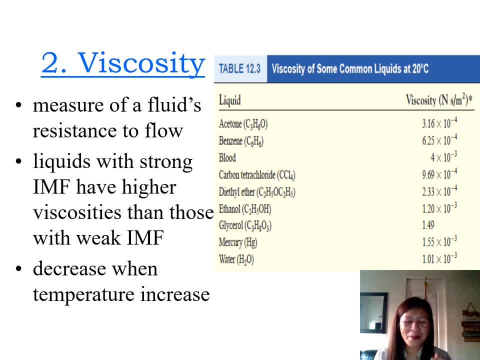 So it's like yung phlegm di ba, Pagka nahihirapan tayong ilabas pagka may phlegma tayo Kasi masyadong viscous ang phlegm, Masyado siyang resistant to flow. 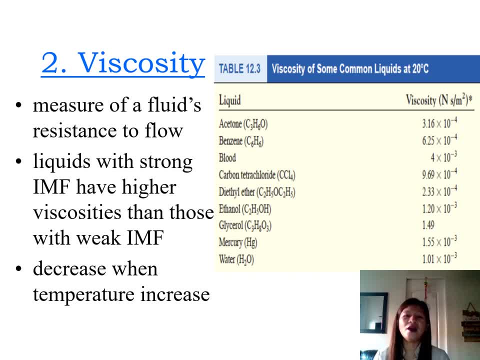 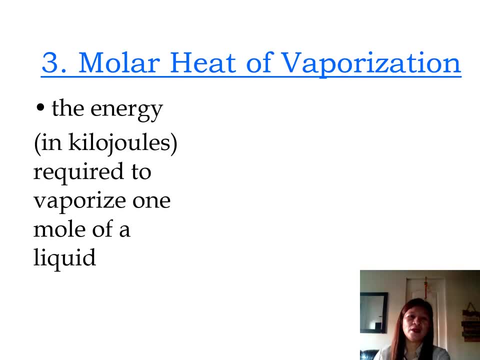 It is highly viscous when compared to typical liquid Like water, alcohol or acetone. So that's what we mean by viscosity. Another property of liquid is the molar heat of vaporization. This is defined as the ability or the energy in kilojoules required to vaporize one mole or to turn one mole of a liquid to gas. 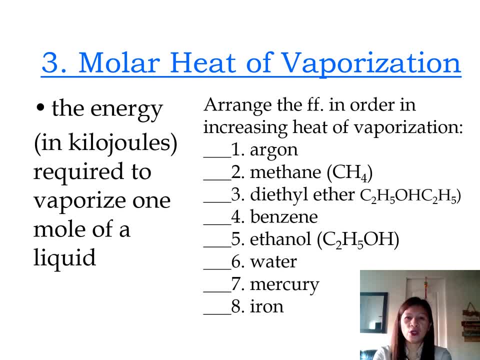 Let's arrange the following in order of increasing heat of vaporization. Again, heat of vaporization is the energy necessary to vaporize a liquid. We have argon. Argon is one of the noble gases, So this is a nonpolar molecule. 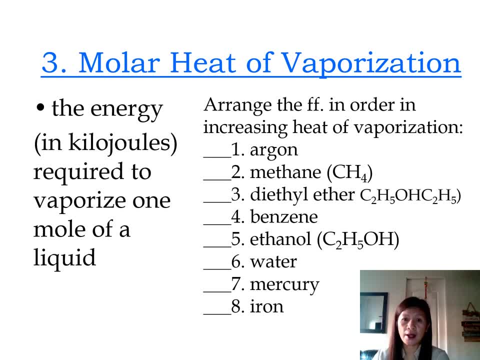 Methane is also nonpolar. Diethyl ether is also nonpolar. Benzene nonpolar. Ethanol polar Water, polar Mercury metallic And iron also metallic. So in terms of strength of intermolecular heat, 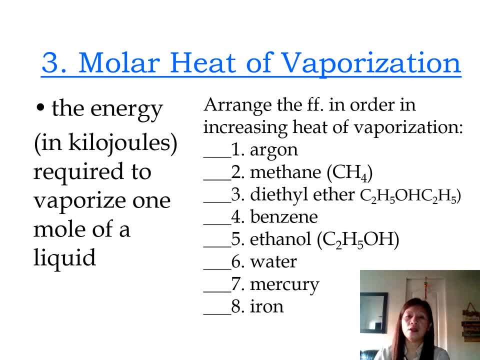 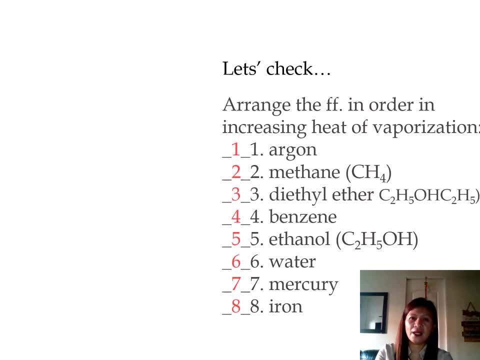 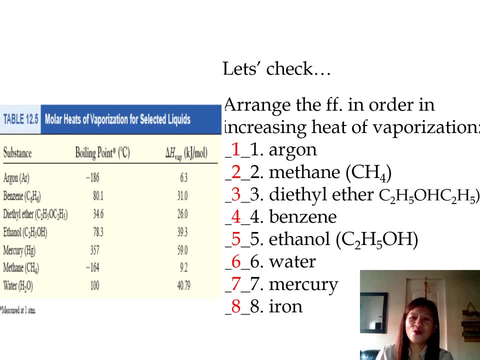 So, in terms of strength of intermolecular forces, you can determine the order in terms of heat of vaporization And the answer is this: So parang naka-arrange na siya. So, in terms of heat of vaporization, this is increasing from argon to iron. 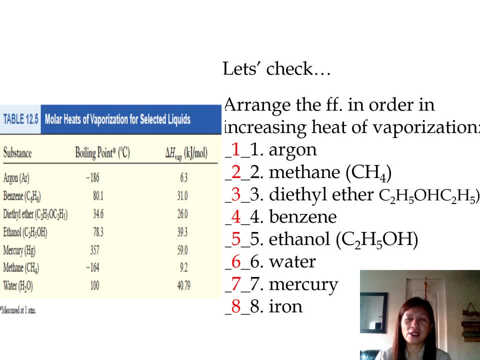 So take note of the strength of intermolecular forces. Sabi nga natin pag nonpolar weak ang intermolecular forces. The type of IMF is London, or dispersion forces. The weakest of all intermolecular forces, Hydrogen bond is the strongest. 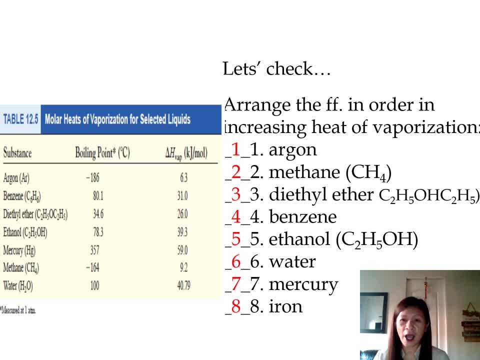 But pag meron kang involved na ionic, syempre stronger ang ionic, Much stronger kung metallic. So that what accounts for the order here? Increasing heat of vaporization, The strength of intermolecular forces, As we can see here. 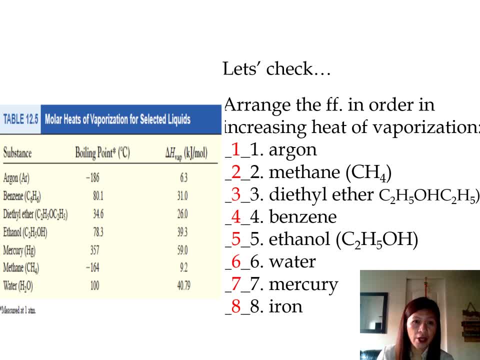 We have argon with 6.3 heat of vaporization, compared to water 40.79.. Argon is nonpolar, Water is polar. So between nonpolar and polar, polar has stronger intermolecular force, So that accounts for the big difference. 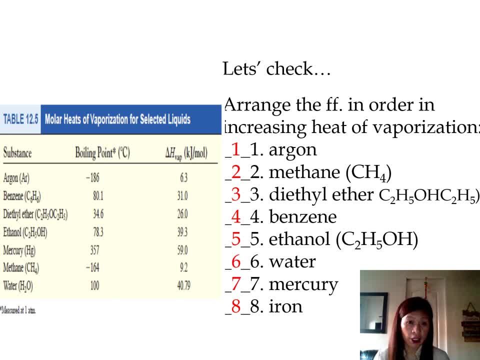 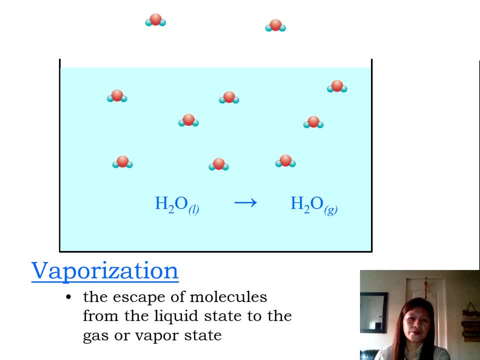 Between the heat of vaporization of argon and water. Okay, When molecules escape from the liquid state to form gas or vapor, This is called vaporization. So to vaporize one mole is to apply certain amount of energy for the molar heat of vaporization. 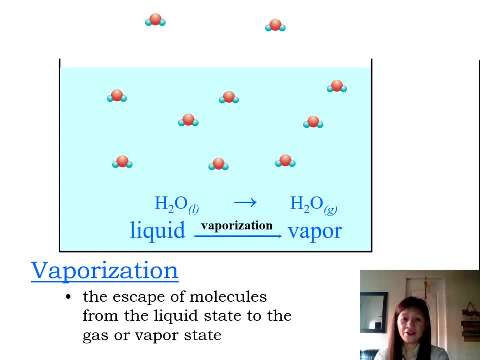 The process of turning liquid to vapor is vaporization And vice versa. We have vapor to liquid, We have condensation. Once liquid molecules escape to become vapor, They begin to exert vapor pressure. Vapor pressure is the pressure exerted by a vapor in equilibrium with its liquid. 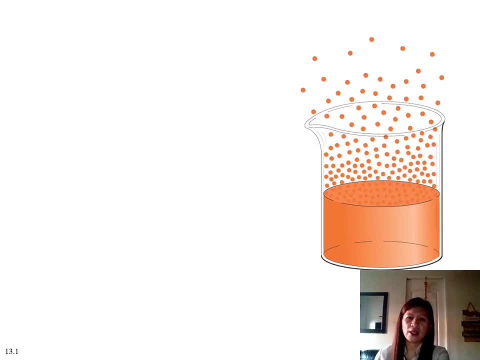 Let's take a look at this illustration. Okay, Let's take a look at this illustration. So we have a container here that is open. So what happens when you leave a liquid in an open space after, let's say, several hours or even days? 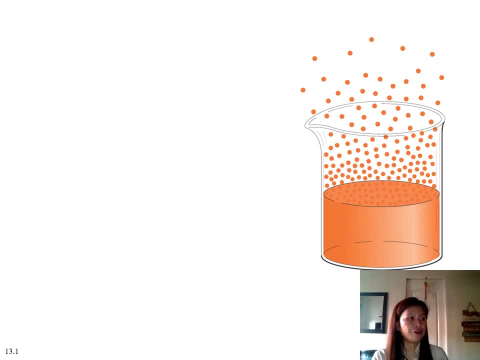 Isn't it like this water that we left? after one week, For example, we left and when we came back it's gone, Because even at room temperature, water molecules vaporize. So because it's not, Room temperature is not 0 degrees Celsius. 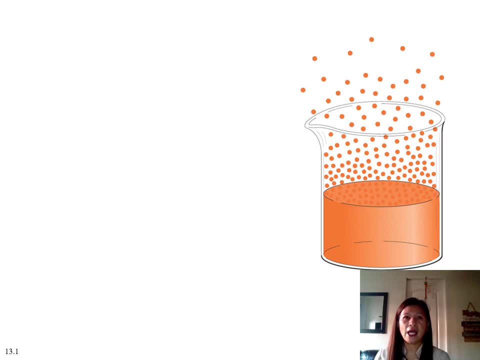 It's between 20 to 30 degrees Celsius. At that point we have what we call volatility. The liquid doesn't need to be heated to a certain temperature before it vaporizes, So naturally, molecules escape from the liquid state to become vapor. 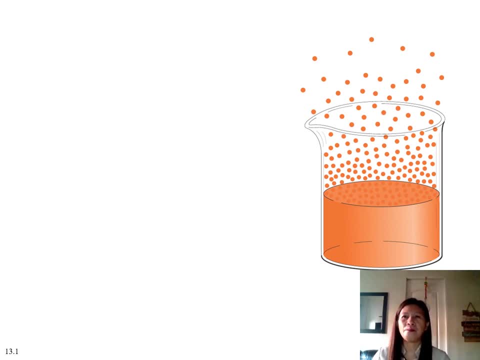 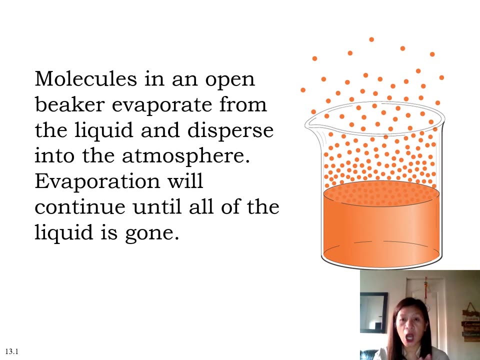 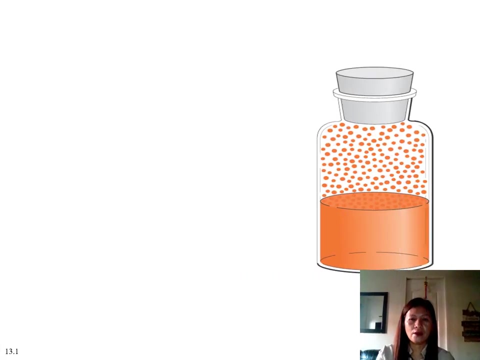 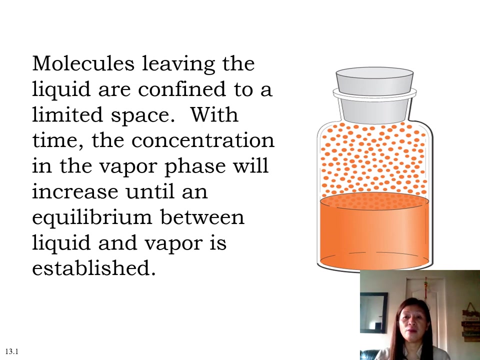 So that's what happens when the level drops. Once we leave a liquid in an open space, Because water molecules are escaping, They escape, they vaporize until such time that all the molecules have escaped the liquid state. On the other hand, if the container is closed, even if it's still vaporizing, the level won't go down or it won't run out. 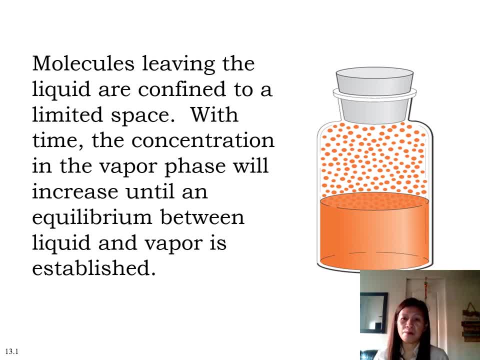 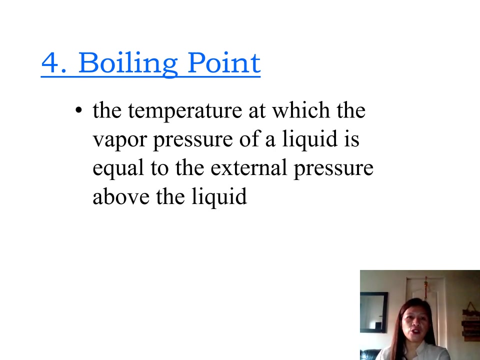 Because water molecules are escaping. Water molecules are escaping, They vaporize, but they also return. There is equilibrium between vaporization and condensation. in this situation, In connection to vapor pressure, let's have the fourth property of liquid, the boiling point. 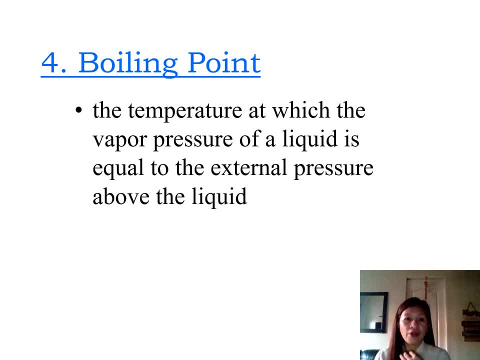 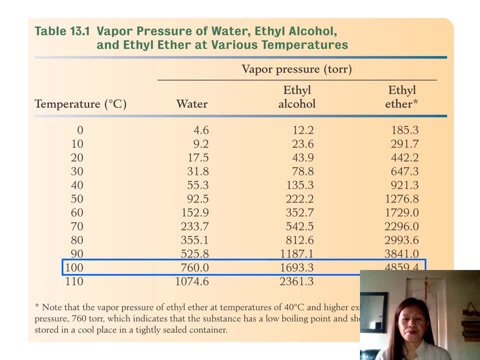 the vapor pressures of the three differ. So among the three, aling yung pinaka mabilis magbo-boil, Since the atmospheric pressure is 760 T. mas mabilis magboil ang ethyl ether kasi mabilis. 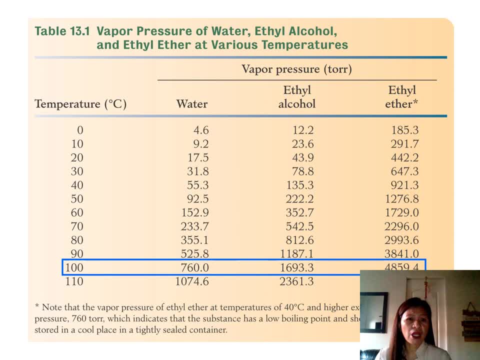 niyang mariritch yung same atmospheric pressure. Water requires 100 degrees Celsius para maritch na yung 760 T and boil, while ethyl ether requires much less energy to reach that temperature, to reach that atmospheric pressure, for its vapor pressure to become equal with the atmospheric. 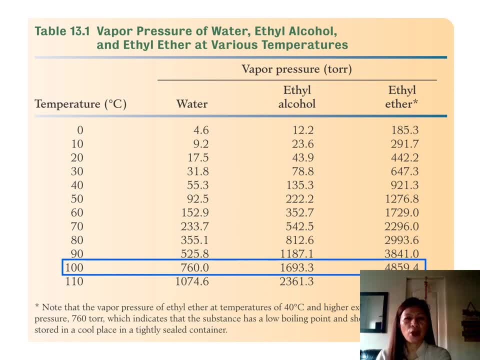 pressure and boil. So when you compare the boiling points, of the three aling sa kanila, yung pinaka mataas Of course that of water at ang pinaka mababa ay ang sa ethyl ether. So again, anong relationship ng boiling point, vapor pressure, sa intermolecular forces? 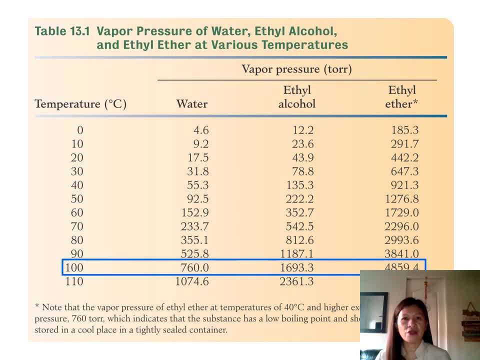 The stronger the intermolecular forces, the higher the amount of energy required to vaporize. For a liquid to vaporize we need energy. So the greater amount of energy required to vaporize, the greater the boiling point. So mas ang pagtaas ng vapor pressure ay may kinalaman sa amount of vaporization, Mas mabilis mag-vaporize. 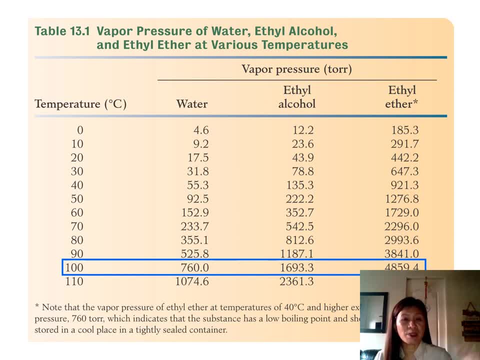 yung liquid mas mabilis tataas, yung vapor pressure mas mabilis mariritch ang same atmospheric pressure at mag-boil. So kung mababa mahina yung intermolecular force mabilis mag-vaporize. 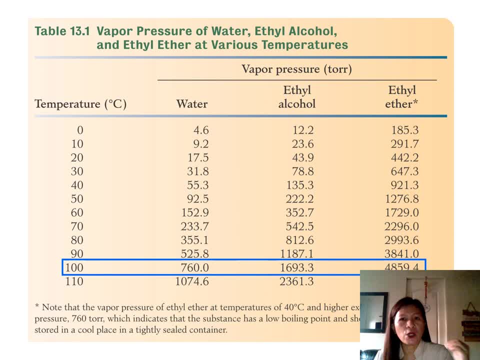 mag-escape from the liquid state, yung mga molecules mas mabilis mag-accumulate or tataas, yung vapor pressure mas mabilis mariritch ang same atmospheric pressure at magboil. So kung mababa mahina yung. 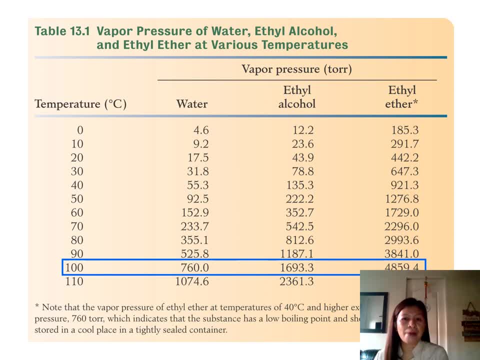 atmospheric pressure and the liquid will boil faster. So among the three, water, ethyl alcohol and ethyl ether is strongest in water and therefore it requires highest amount of energy to boil. Ethyl ether requires the smallest amount of energy to reach the atmospheric pressure. 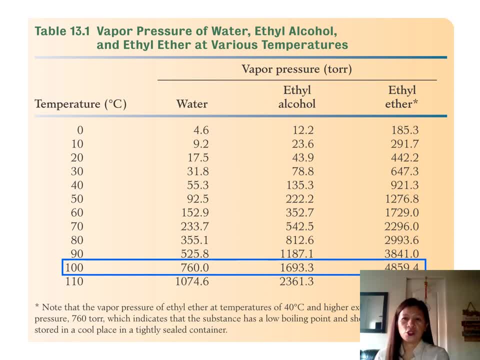 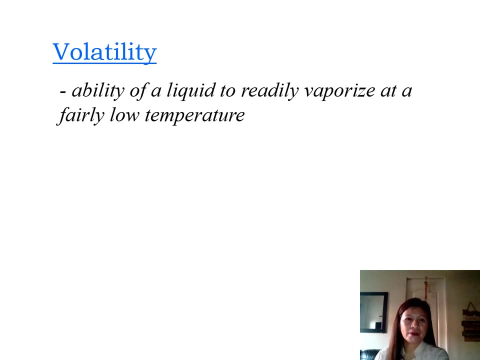 and boil, So weakest attraction in ethyl. ether. strongest attraction in water, So highest the boiling point for water, lowest boiling point for ethyl. Another property is volatility: ability of a liquid to readily vaporize at a fairly low temperature, for example 20 degrees Celsius. 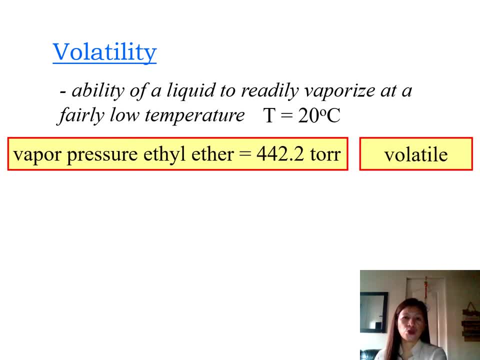 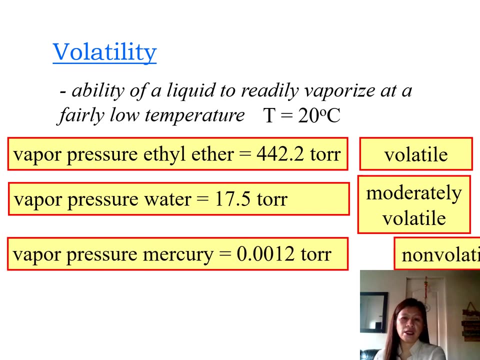 So vapor pressure of ethyl ether is 442.2 Torer, So ethyl ether is volatile. uh, vapor pressure of water is 17.5 Torer. It's only moderately volatile and mercury is nonvolatile. Can you explain the following in terms of IMF? 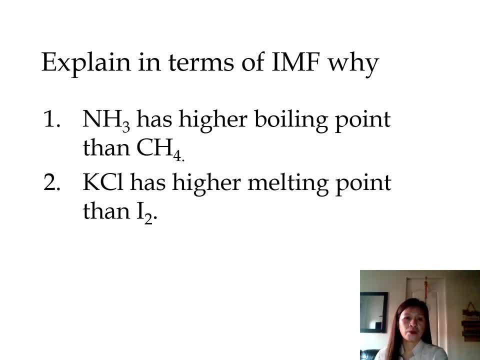 Ammonia has higher boiling point than methane. Ammonia is a polar molecule and therefore the type of intermolecular force is dipole-dipole. Methane is non-polar and therefore dispersion Dispersion is weaker than dipole-dipole.